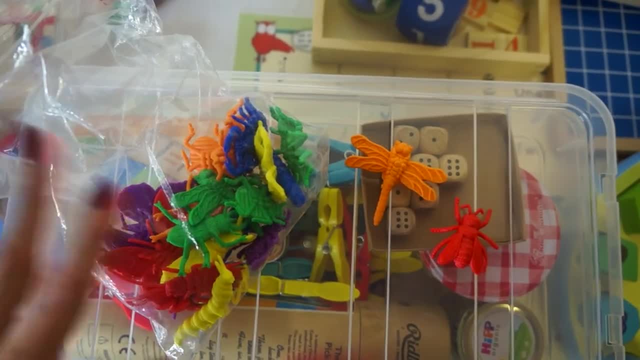 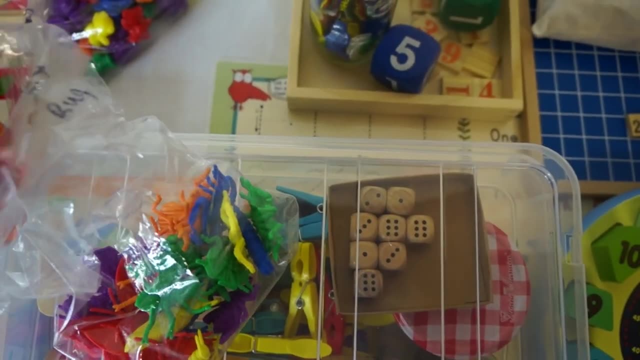 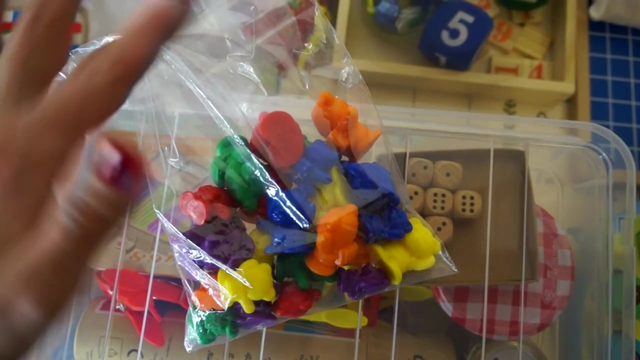 activity. They really like these, So I got these on eBay. actually, There were bugs, there was transport, there was sea creatures, So you can use those for lots of different counting activities. I've also got the bears Now there are lots of these counter bears around on. 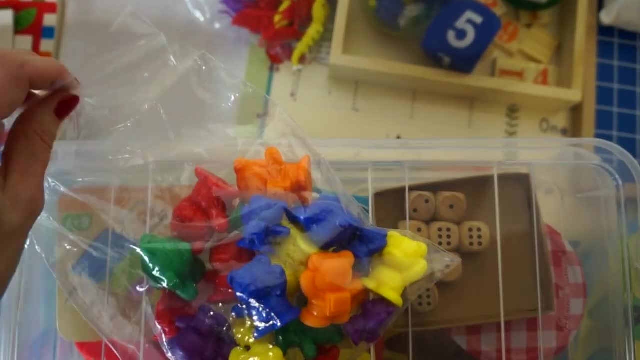 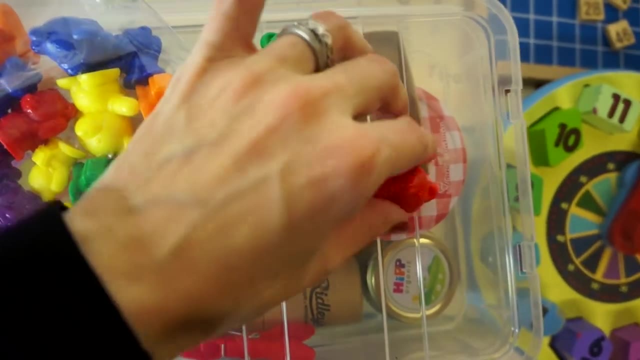 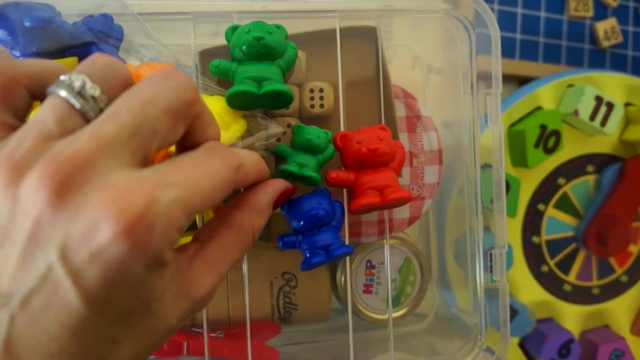 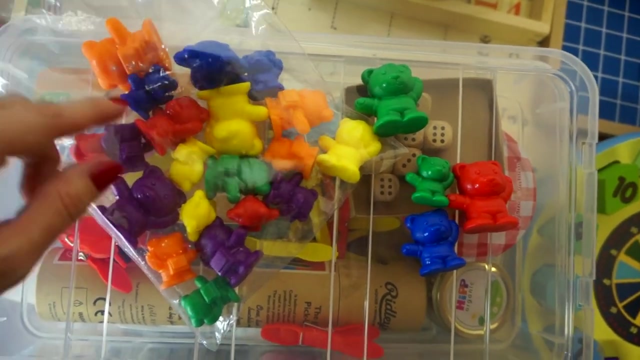 the internet. Some of them are very expensive. These ones are different sizes, So you've got small, medium and large, So you can use these for pattern matching, colour matching, sizing, whatever you like. Again, I have the 24 pack. I think there was a 72 pack. I think these were about a fiver. 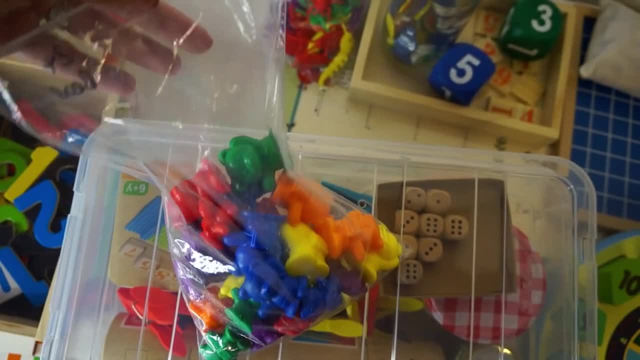 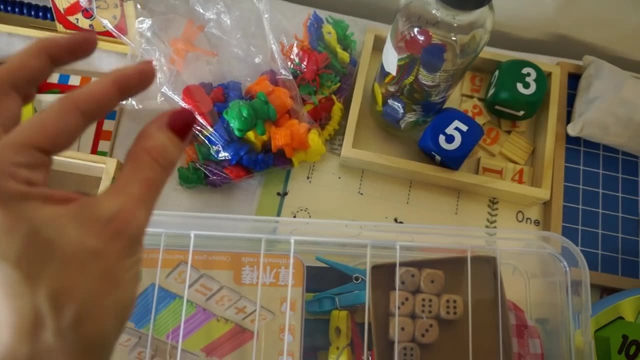 So good price as well. Don't forget, when you're doing counting you can also use things you've got around the house. You can even use cereal. I've seen lots of cheerio activities where the child counts out the cheerios or beans- Not baked beans- That could get. 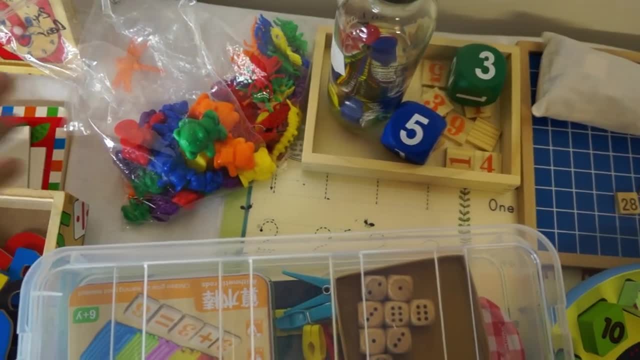 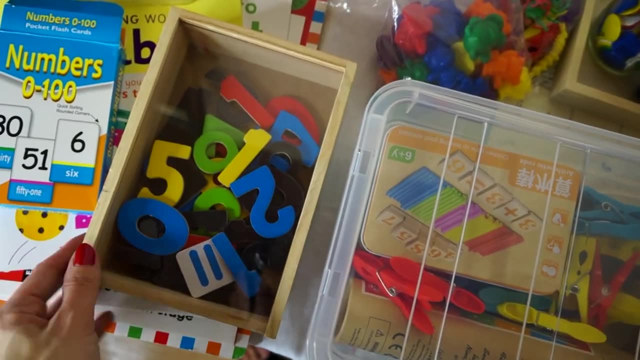 a little bit messy. So, anything you like, You don't have to go out and buy counters. You could have things around the house, So that's nice and easy to use. Then, moving on to actual numbers. So I've got this box here. This was Melissa and Doug. 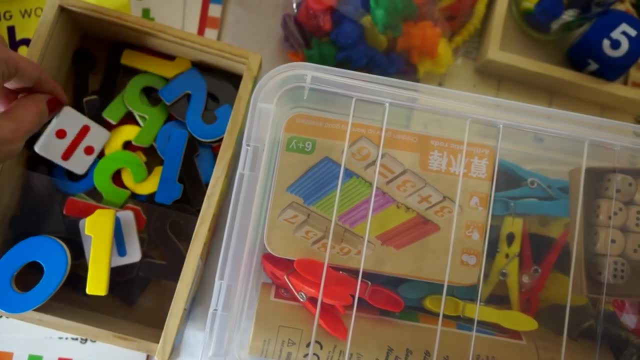 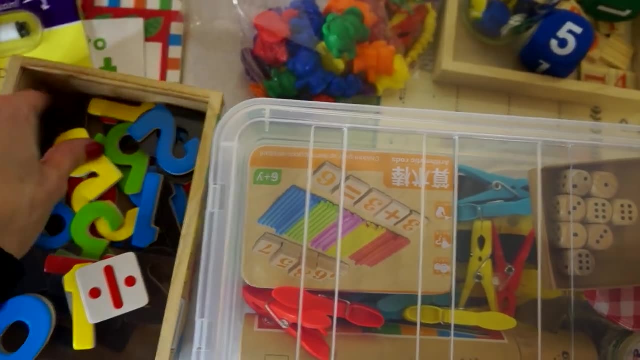 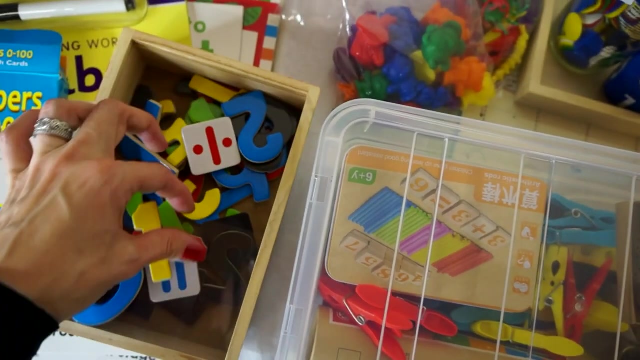 These are magnetic numbers. I think you've got 0 to 9, and then obviously you can make up the numbers 10 and so on, And they've also got all the symbols for your multiplication, your division and so on. But these are really nice. I've also got some plastic magnetic numbers, So anything you 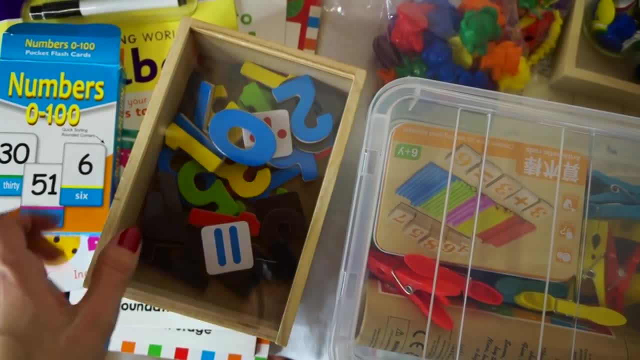 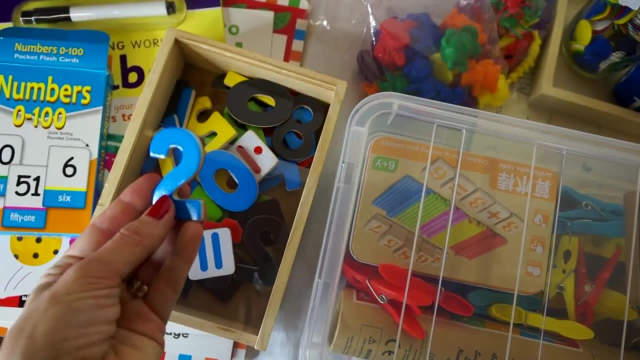 like, and then you can stick them on the fridge, You can stick them onto a whiteboard or you can just pop them onto a piece of paper Maybe, write the numbers and say: can you match number two with number two on the paper, and so on, And it comes in a nice little handy box there. 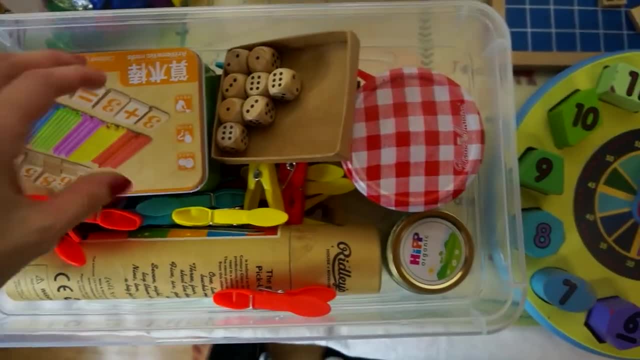 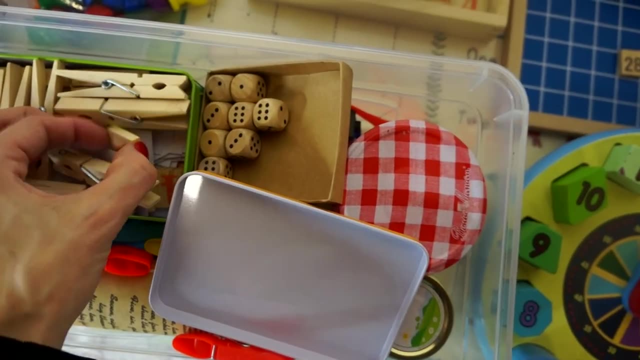 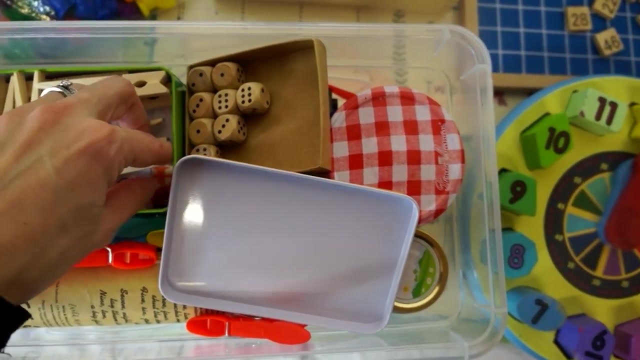 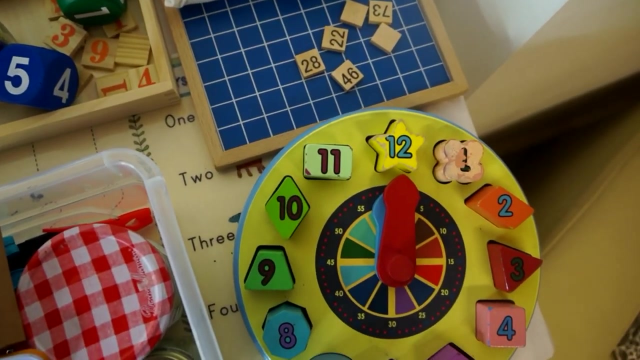 as well. I've also got other numbers in here. This is my sort of maths Resources box, So I've got these little numbers. What is that? Oh, that's the less than sign. I've got some little numbers on wooden tiles here, And I've also got this. I know this. 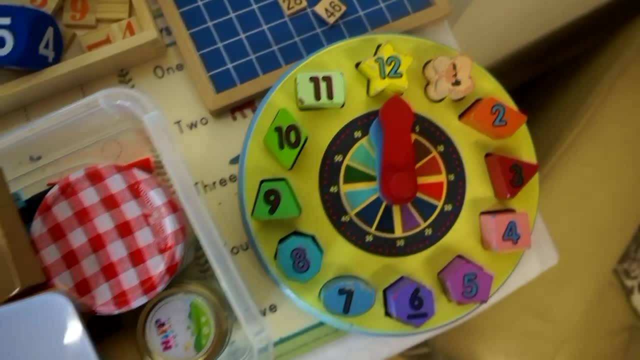 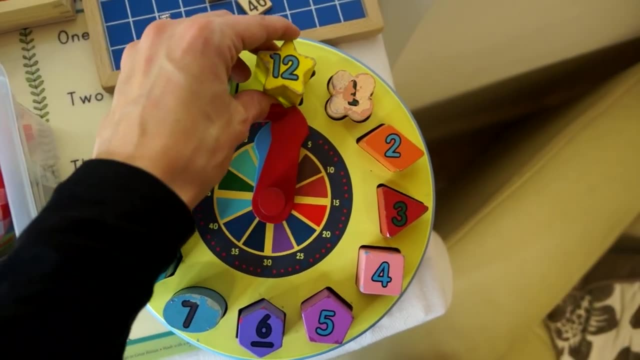 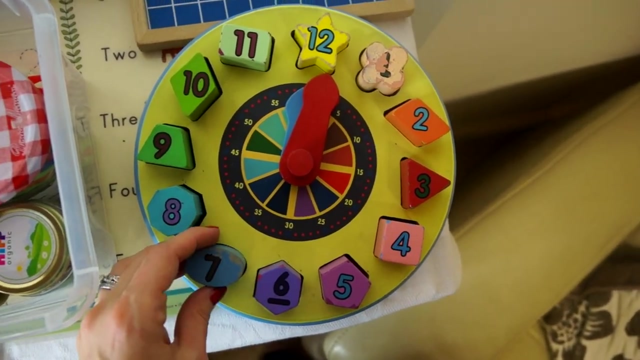 is a clock and you might not necessarily be doing the time with your child, But these chunky numbers are nice to use for number recognition, Shape recognition, So that's quite nice. if you've got anything like that, That kind of toy or game, You could use that for your activities. 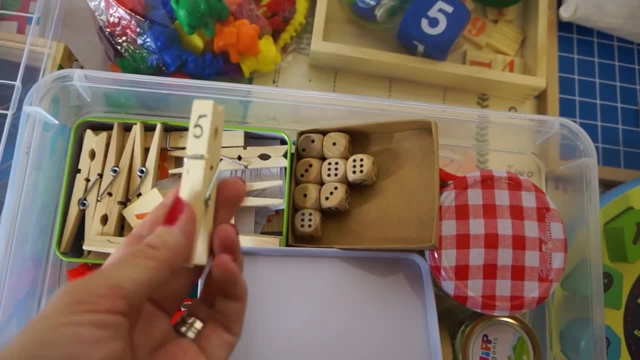 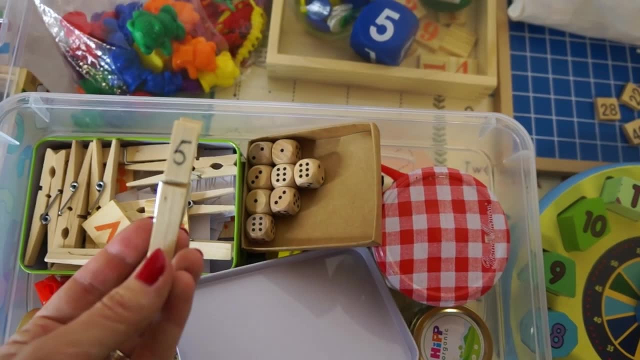 I also have these wooden pegs with numbers on. Basically I bought the wooden pegs for like a pound And I just popped the numbers on there. I think I did 1 to 10.. But you could do 1 to 20, 1 to 50, depending on how many pegs you have. And these are quite nice for. 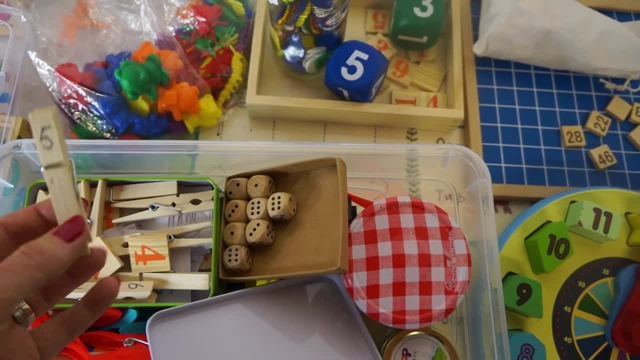 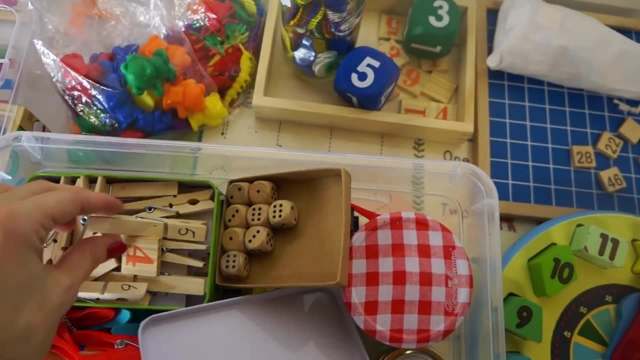 simple games. So you could have a piece of paper with the different numbers on and they could be a peg, The peg onto the correct number. Lots of different activities you can do with those. And then I've got these fantastic number dice. These I got off Amazon- They were from the 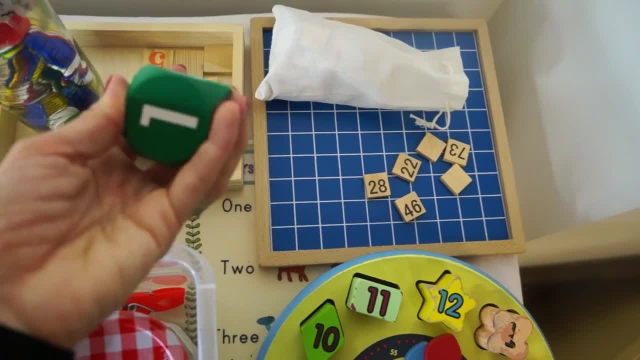 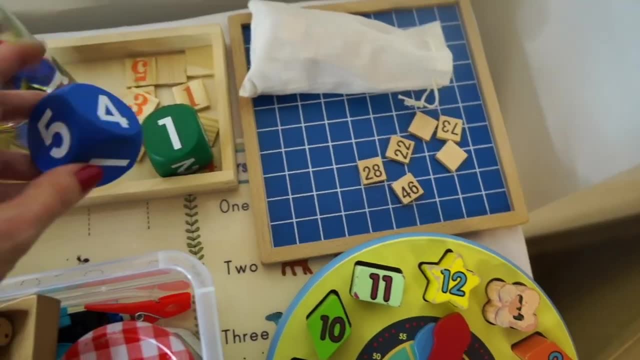 Learning Resources Company. There's two in a pack. They are nice and large, Made of foam, So a really nice ergonomic fit for young children. And what we do is we sort of roll the dice and I'll say what number is that? Oh, my son will go, it's number 5.. Let's take 5 steps. 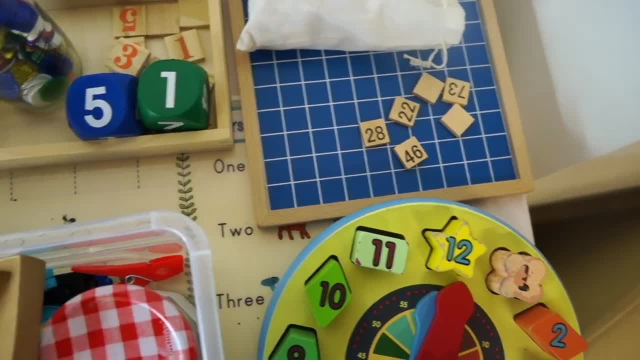 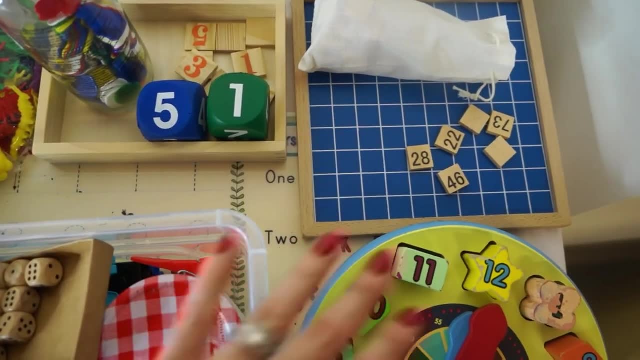 forward. So if you've got a piece of paper, that's not a big deal. You can put the number on it, Or you can put the number on the foam mat, Or you can put those foam mats down That have got the different numbers on, And whatever number the dice lands on, they have to jump. 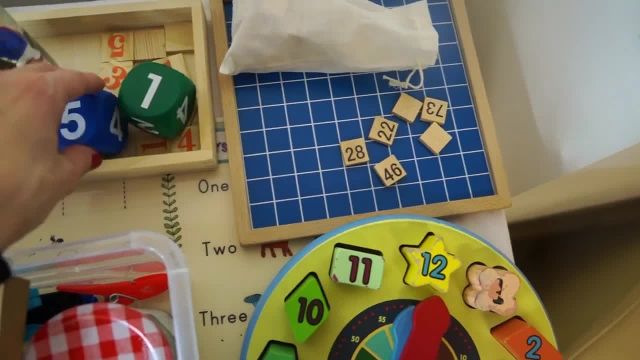 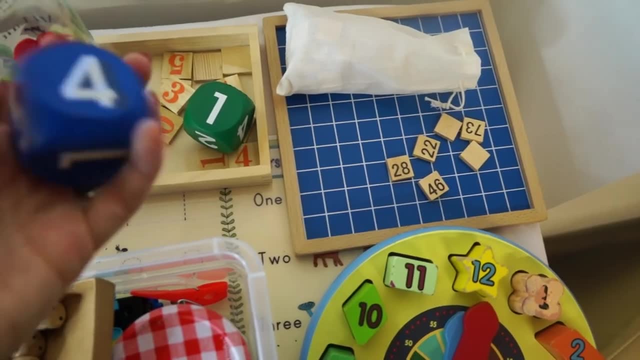 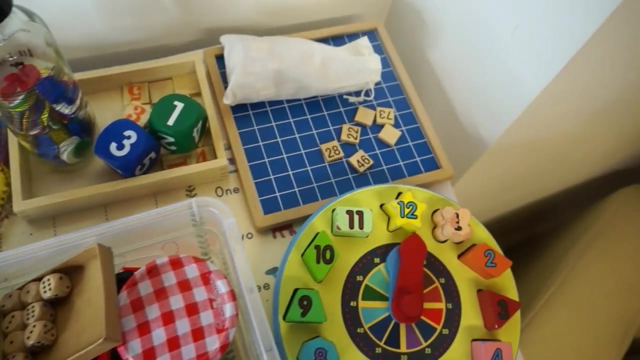 to that foam tile with that correct number on. There's lots of different activities you can do with these number dice as well. I've also just bought some foam dice with the dots on. So not necessarily the number, It's the number of dots. So depending on where your 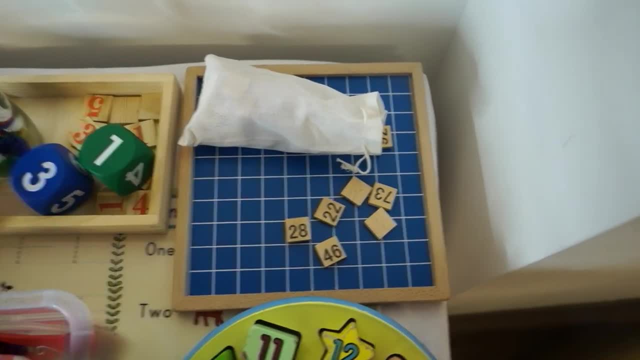 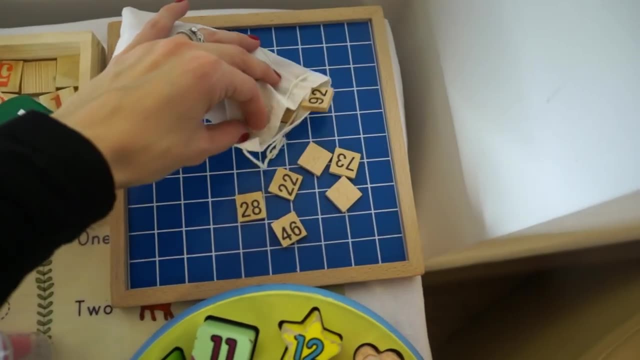 got this Montessori number board, but it is a mini version of the Montessori number board. when I bought it I thought it was a larger one, but no matter, it does exactly the same thing. it comes with the tiles 1 to 100. I don't do 1 to. 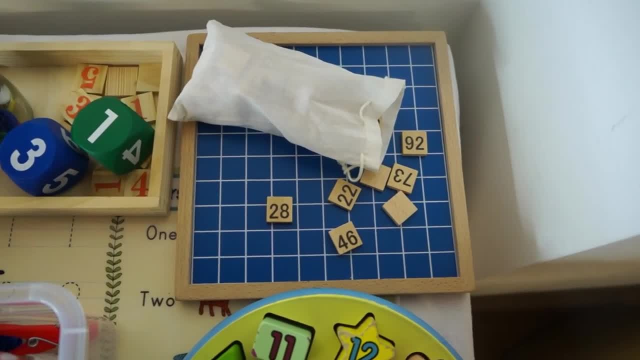 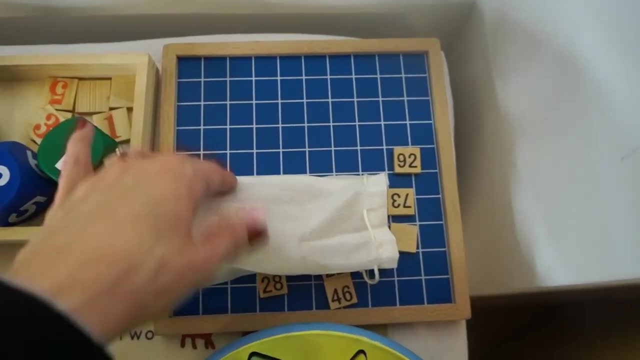 100 with my children because they're still young- my eldest is nearly 4 and my younger one is 2- so we tend to just do you know the numbers 1 to 10 or 1 to 20. you can do them diagonally or you know straight across, however you like. this is. 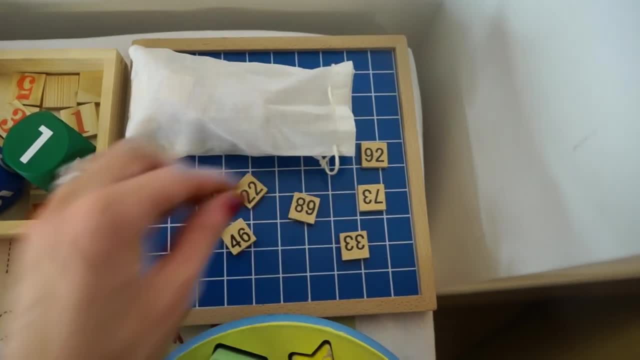 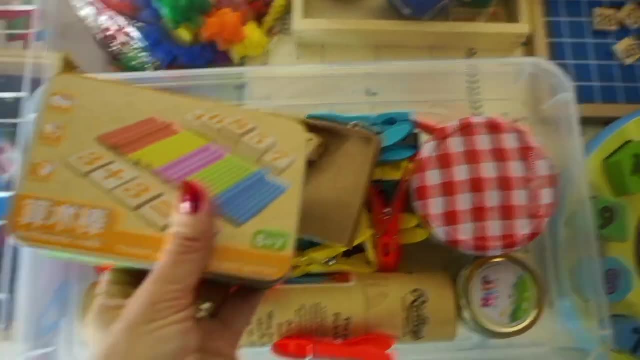 always a nice learning resource to have in your home. so let's take a look at what else I've got in the shoe box. so, um, this I actually bought online, so it had the little wooden tiles in there. I just added the pegs in there as well, so had 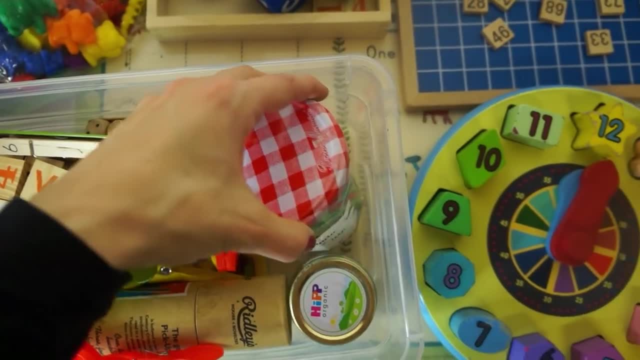 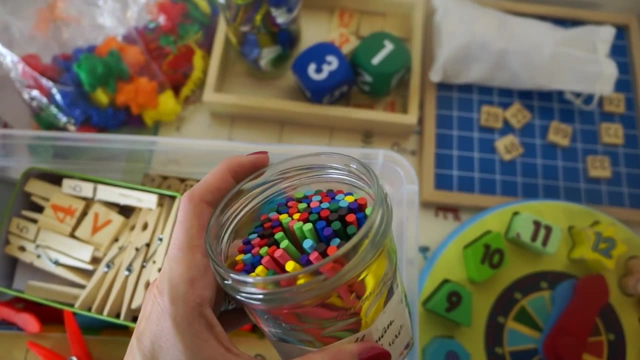 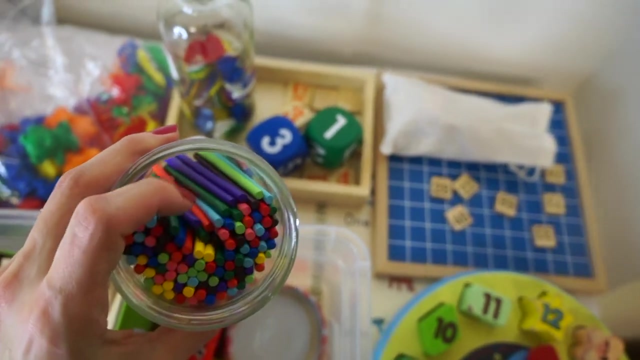 the little wooden tiles. and then it also came with these rods which I popped in this jam jar, because when I tipped out this little box I then couldn't get everything back in this. I popped them in here again. you can do different activities with these, you know. 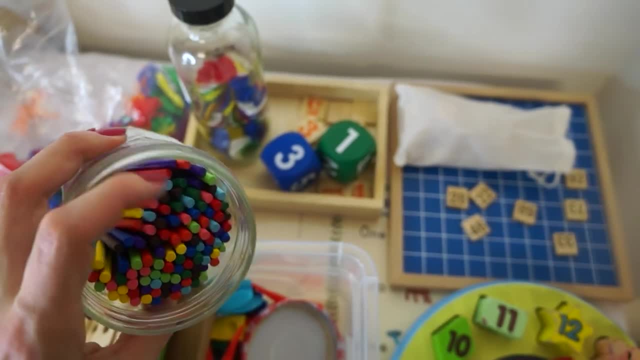 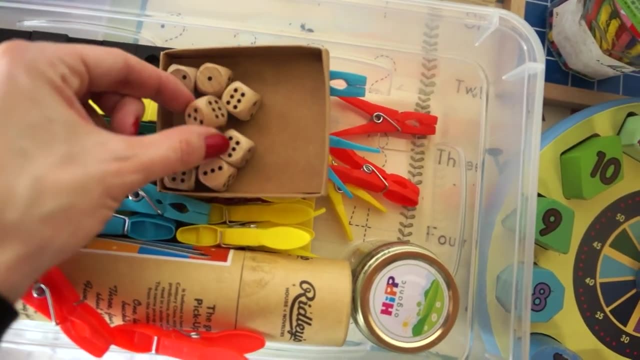 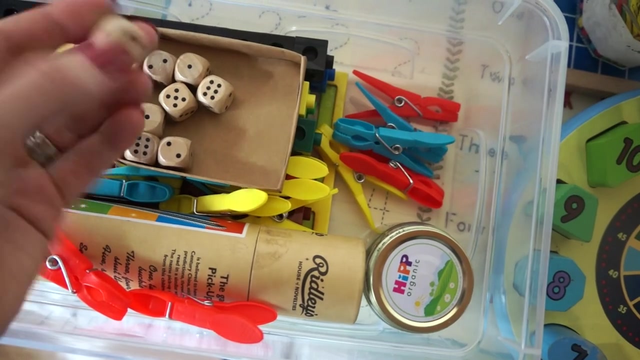 you can roll dice, have a number and then lay out the number of rods, and they're also different colors, so that's quite nice. I've also got smaller wooden dice. I wouldn't advise you to use these, obviously, with small children. even my two-year-old still likes to pop everything in his mouth, but these came. 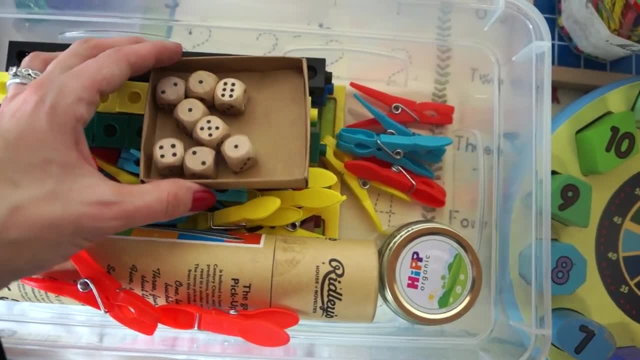 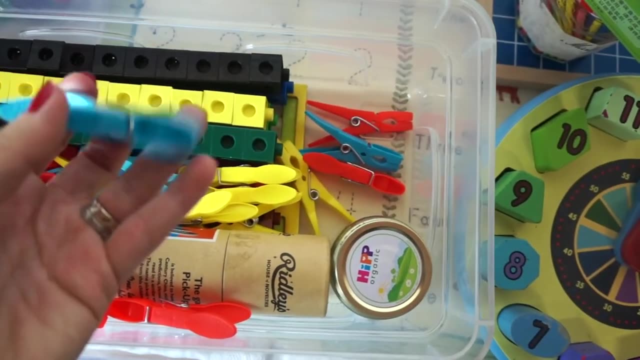 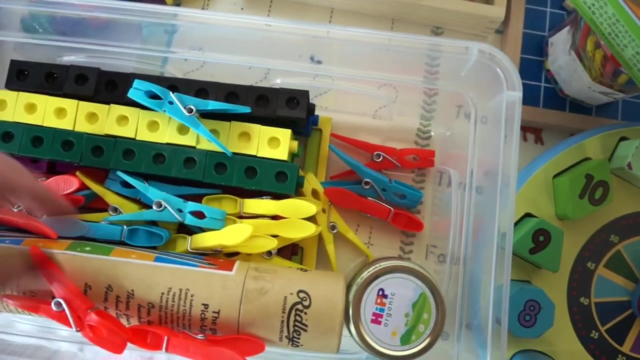 in a pack and I thought perhaps when we were playing other games they might be useful later on. so I've also just got some normal colored plastic pegs again. you can do whatever number activity with those. can you find four blue pegs? can you find three red pegs, or can you peg them to the washing line or whatever? 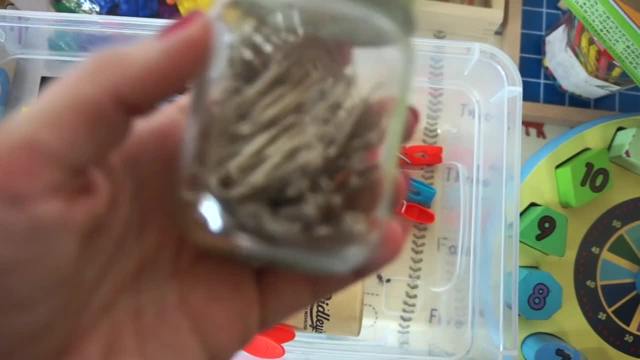 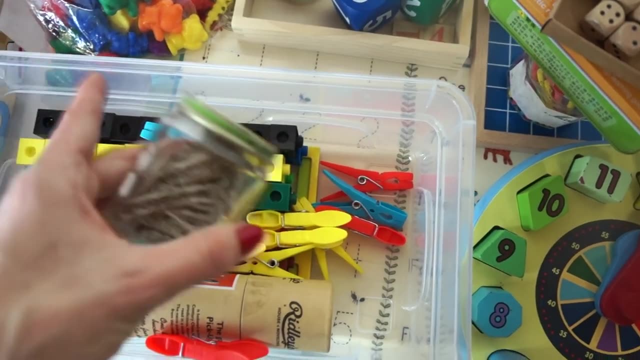 that's quite nice. all other counters I've got paper clips. so actually I do have a an activity that has different pictures with different numbered paper clips. so my son gets out the number of cards and takes theoned out and then has a big game with that. 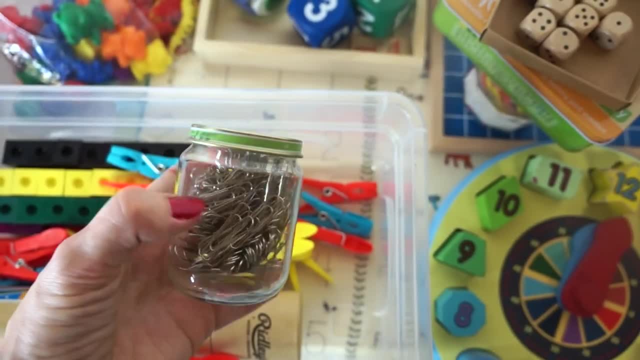 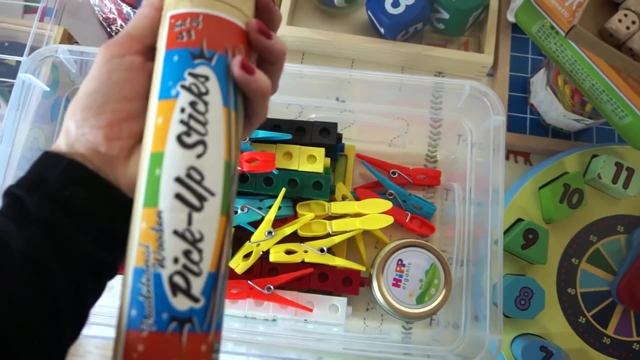 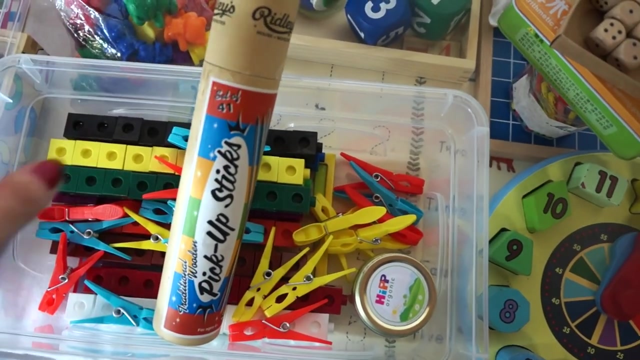 of paper clips and pops them on. i've also got buttons, you. you can use literally anything. so that's that. i've also popped my pickup sticks game in here. this is mathematical, it's logical, it's fine motor skills- lots of um different skills in this one game, so i popped that in here as well. 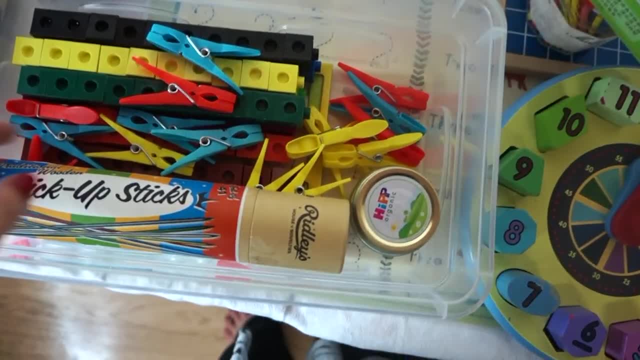 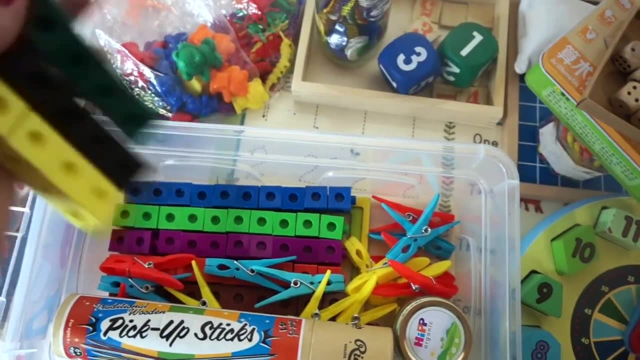 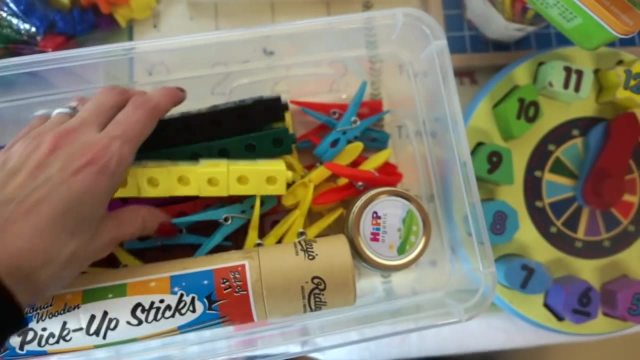 because the children kept opening it and throwing the sticks everywhere, so i thought i'd leave that in here. these are brilliant. um, i never know what the correct name is for these. i think unifix cubes or stacking cubes. i've got a pack of 10 different colors and 10 individual cubes in each one. 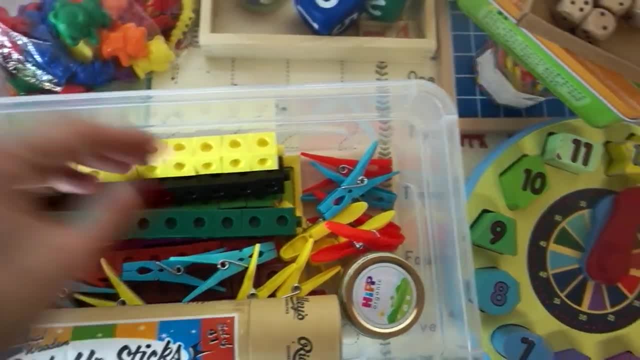 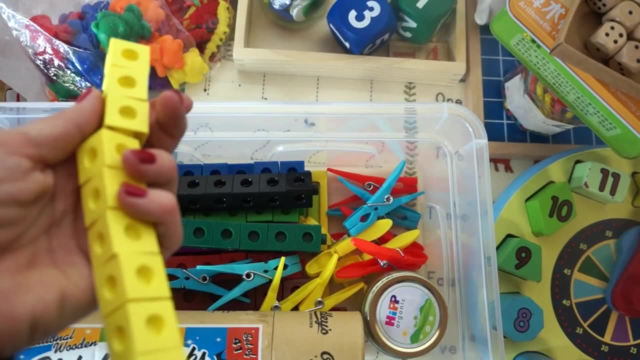 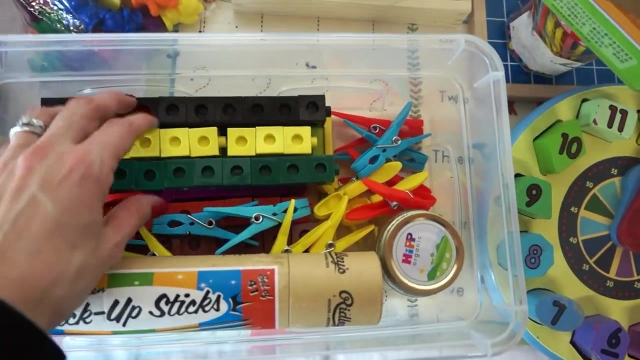 again. this was fairly reasonably priced on amazon. these are excellent for kids to use. you know you can do division, subtraction, multiplication with these. they are an excellent visual learning tool for maths and for colors also. my children like to make shapes with them, so excellent use. this goes way back. people have been using this for many years. 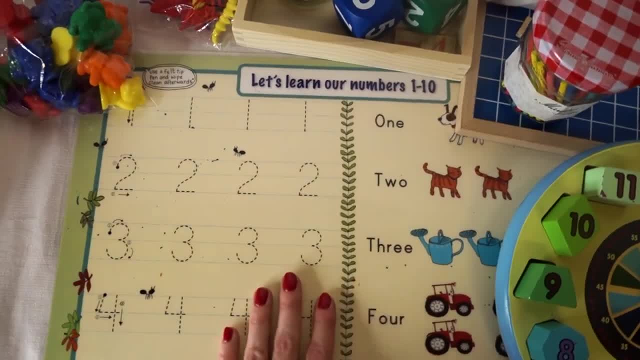 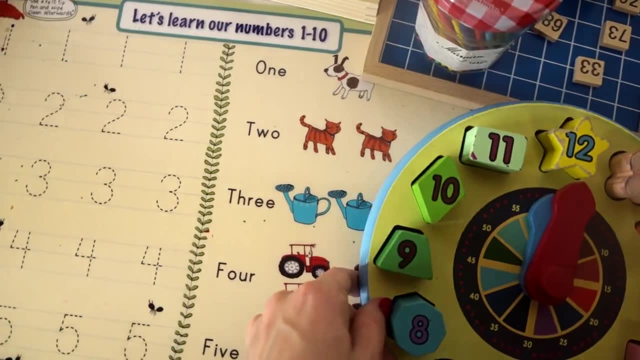 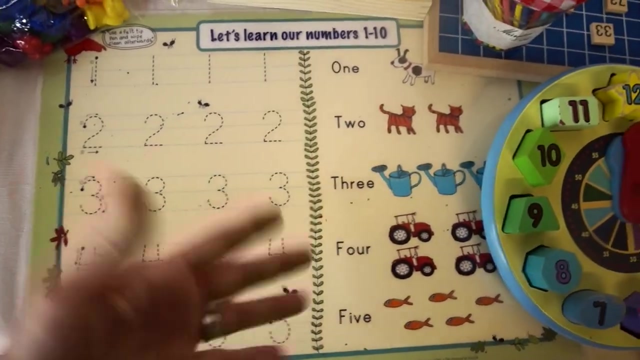 another thing you might like are these mats. um, this is let's learn our numbers one to ten. you can get a dry eraser pen and go over the numbers. it's also got the word one, two, three, four, five. they like to count. i initially was using this as a food mat, so when they 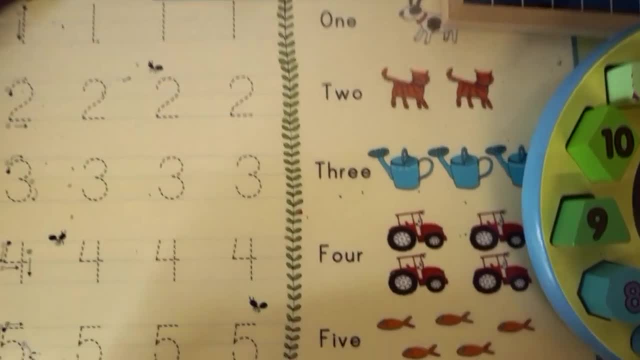 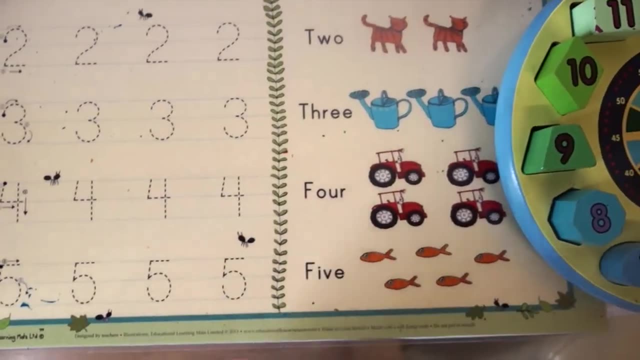 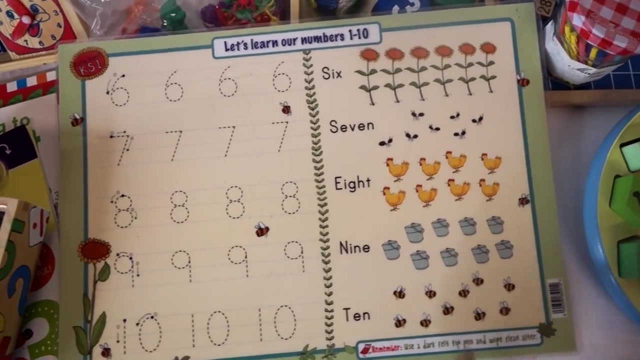 were eating their breakfast. we were looking at the numbers. now i'm using it as a play-doh mat, so it's just a little bit more dirty. um, it's uh, just a laminated mat, and on the back of this one, so it continues with the numbers. these can be quite expensive, especially if you buy them in a. 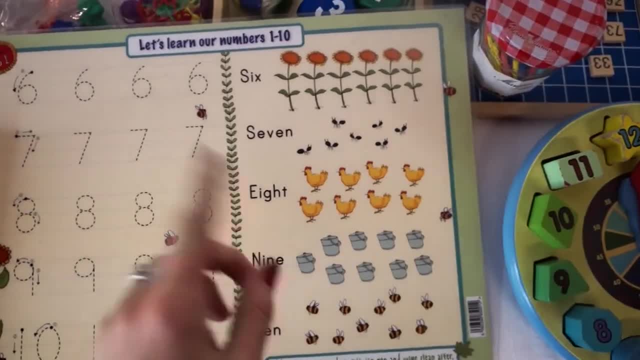 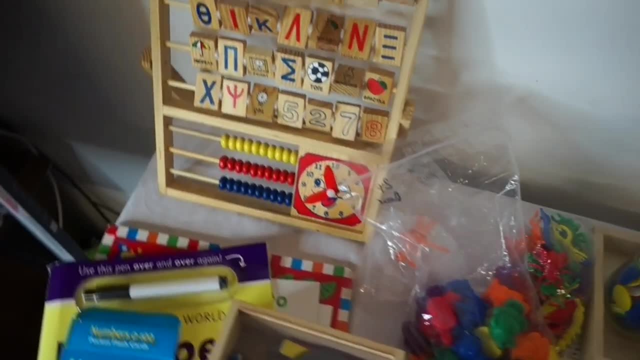 shop that you're better off getting these online again. there's lots of number ones, alphabet ones, but these are really nice just to have as part of your daily routine. you might also want to get yourself an abacus. i've actually ordered a mini abacus now, which will 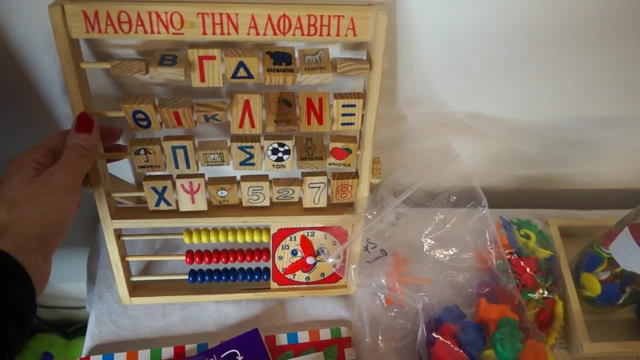 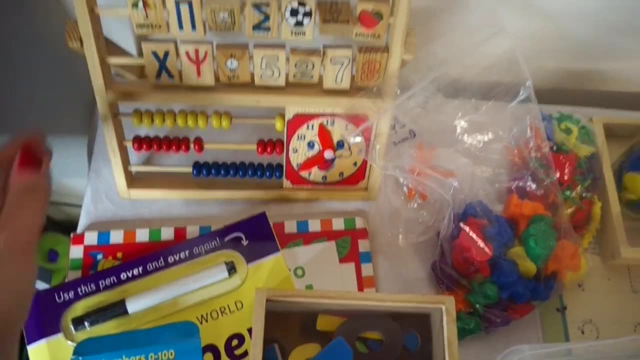 probably be about this size actually. um, this was something we bought from cyprus, so it's got the greek alphabet and little clock and everything. it's just too much for the children at the moment. um, it's. it's too visually stimulating for them to concentrate just on the abacus bit. but, um, i do. 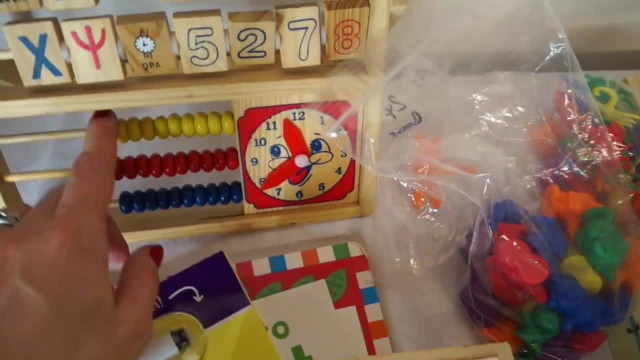 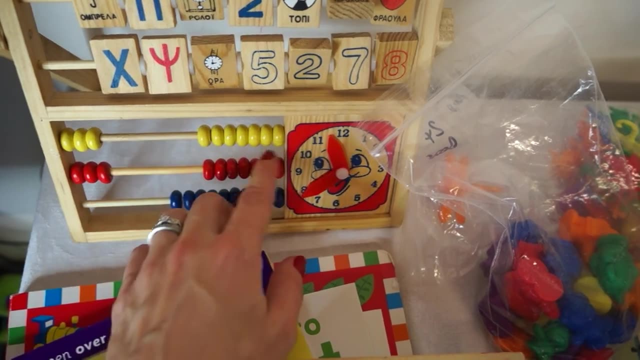 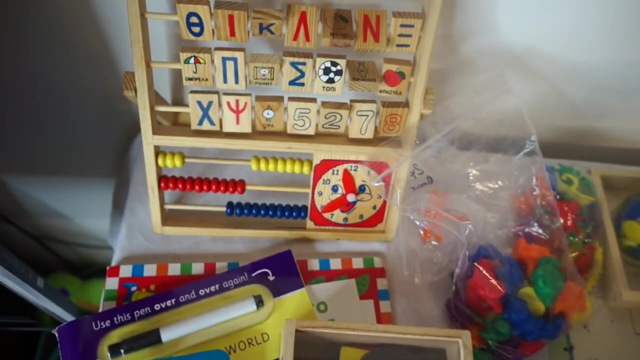 like this one, and it's very good to have an abacus for children so you can say: you know, can you count three across, or can you do five, take away two or whatever. i mean, this is obviously a very traditional mathematical tool and i think every household should have one, even if it's just for therapeutic value. 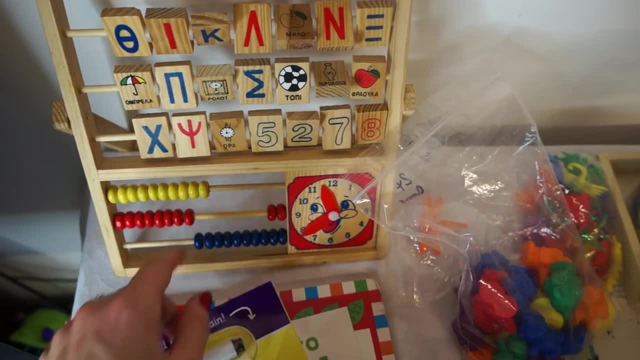 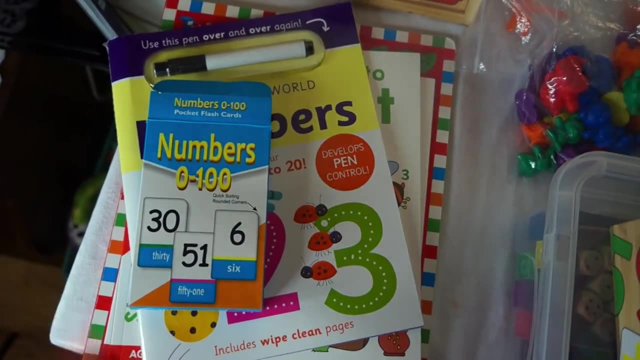 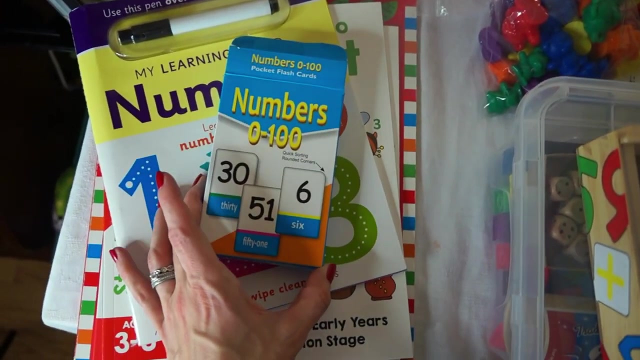 i mean, i just enjoy doing that. ah, so satisfying. okay, now books and flashcards. i showed you all my worksheets in my um learning resources folders, so you can do. you know worksheets and activities like that. flashcards are always excellent. this one is just your basic, nought to. 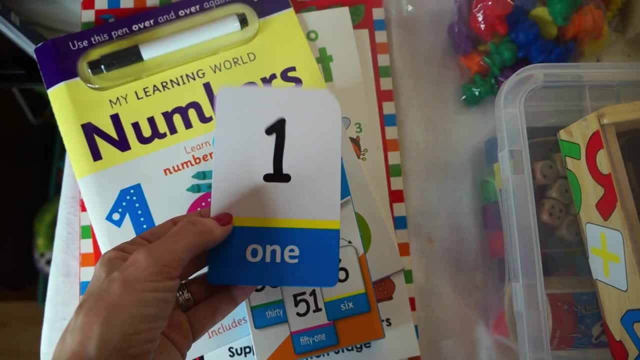 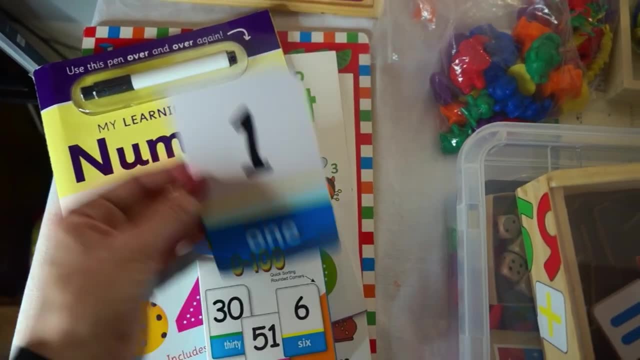 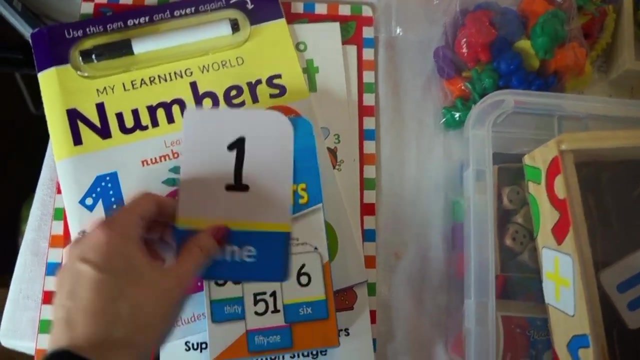 100, very clear number with the word as well. it's got different numbers on the back, so, yeah, don't get confused when you're going one, two and then you're showing the child the number 51, um, but these i just wanted very, very plain, black on white numbers, which was quite 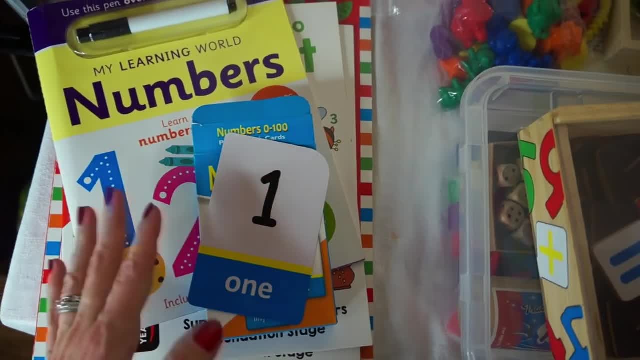 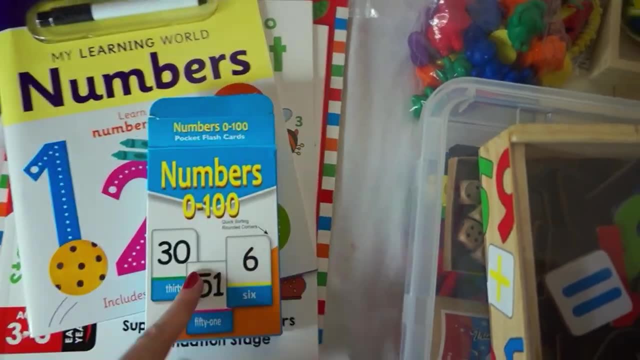 hard to find. actually, with these flashcards, a lot of them have got animals around them and so on, but these are the kind animals around them and so on. but I just want the plain number. so I shall leave all the links, by the way, to everything down below if I can find them, but I'll leave the link to these flashcards as. 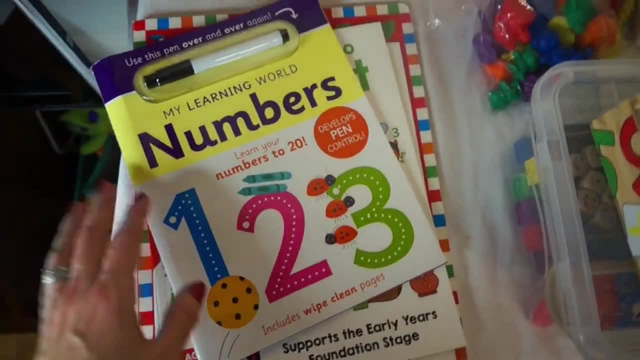 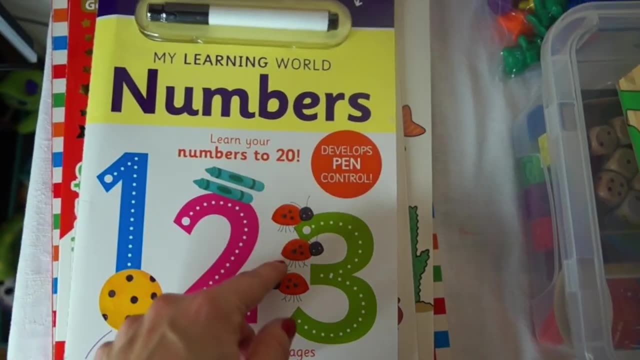 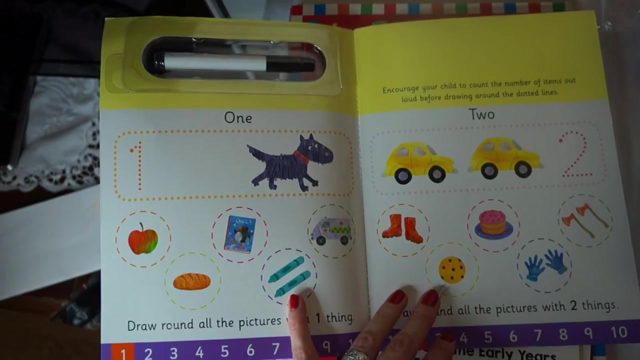 well, now, books. there are loads of fantastic educational books out there. so this is a my learning world numbers: learn your numbers to 20, which includes wipe clean pages and a pen. so let's have a look in here, so you can just ask your child to get the pen and can they trace the? 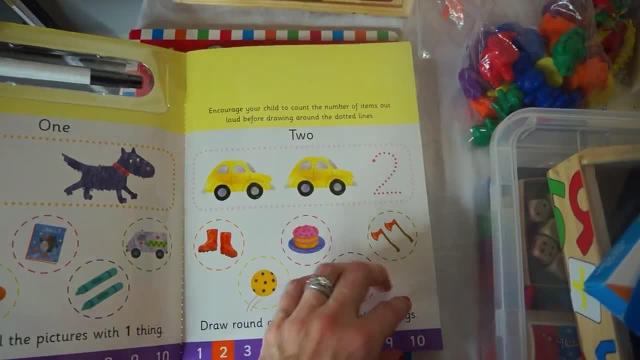 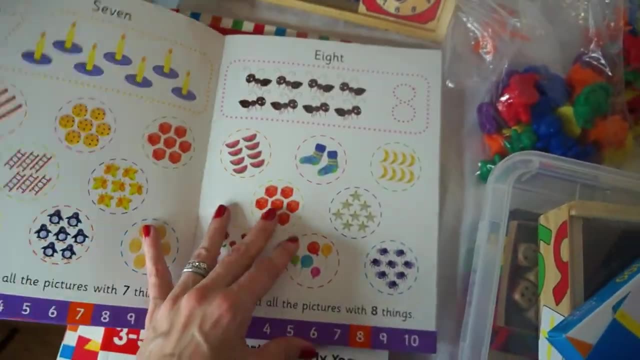 number it says. encourage your child to count the number of items out loud before drawing around the dotted lines, and my sons like to wipe it off as well. so this is just a short book with the numbers 1 to 20, but you could, you know, take that on holiday with you, just a little. 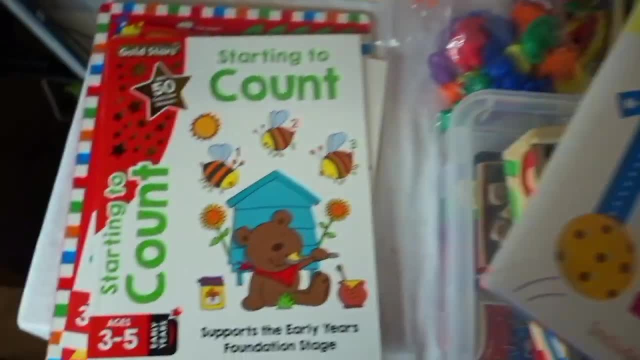 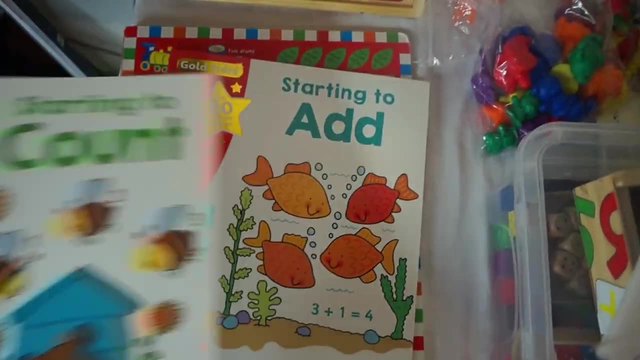 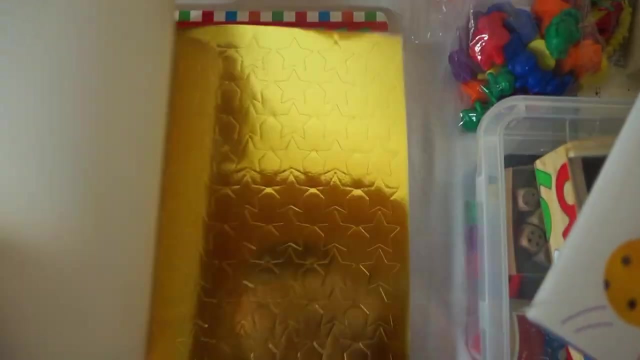 exercise. so there's loads of those out there. I think I've got the one from TK Maxx. then I've got these early years books. I found these in Wilko's and they were about a pound so I quite liked them. I just thought, why not get these? so these you know you'd have to do, obviously, maybe the 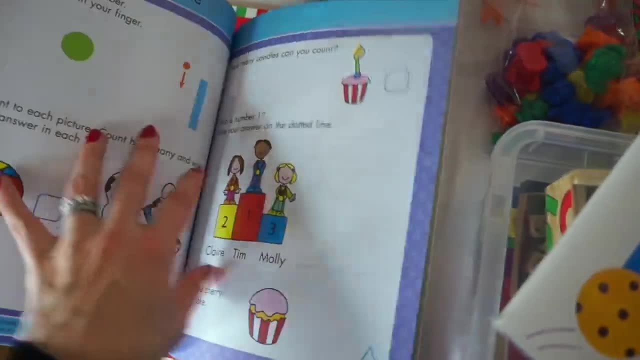 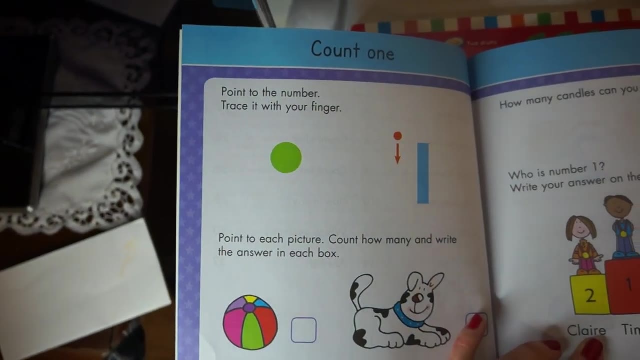 pencil. I would not advise doing with a felt tip, because then you won't be able to go over them again. so let's have a look here. so count one point to the number, trace it with your finger and then point to each picture. count how many and write the answer in each box. 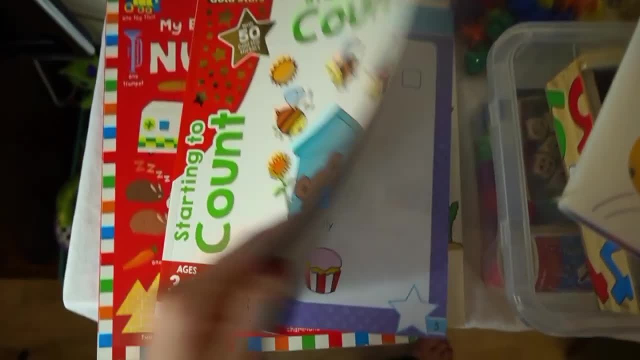 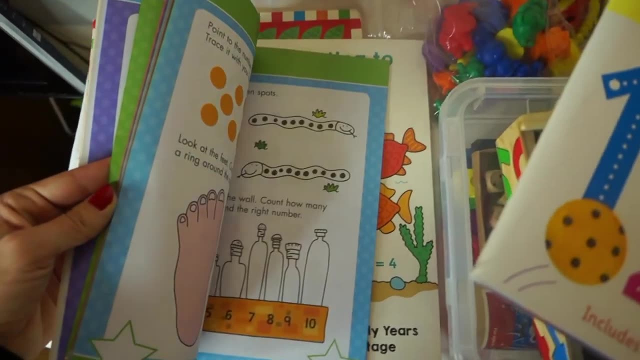 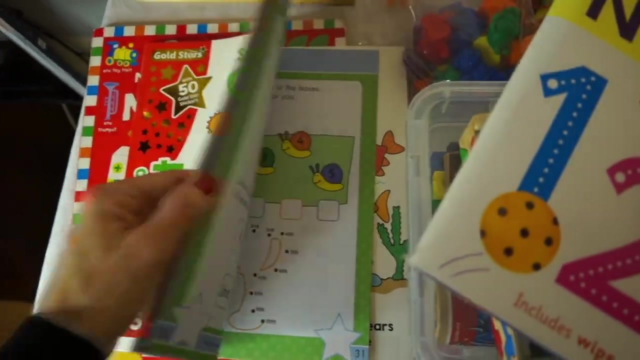 so these are quite nice. this says ages 3 to 5, and I know that when it comes to especially maths, you know they say that just doing worksheets and books isn't enough. you need the tools to make things visually stimulating for them as well and to help engage them. but I think these books are lovely you. 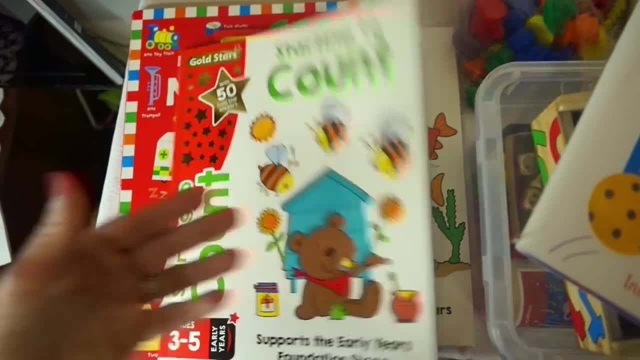 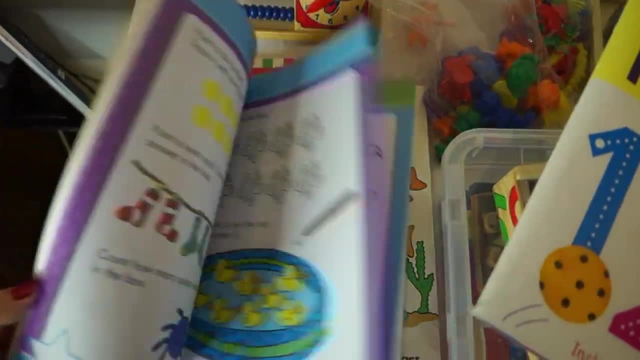 know they're colorful, there are different activities and of course you don't have to do the whole book, you just do maybe one page at a time. this one comes with fifty gold star stickers, as most children do love a good sticker, so that's nice. so I've got the starting to count one and 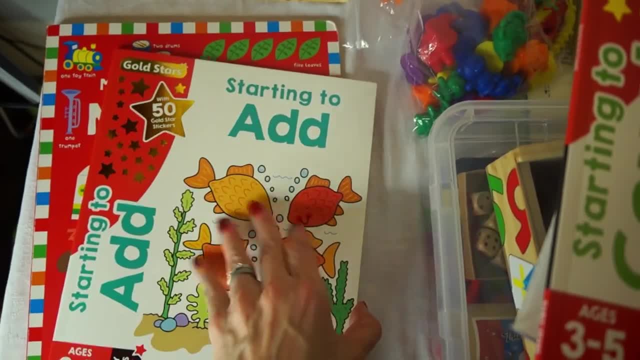 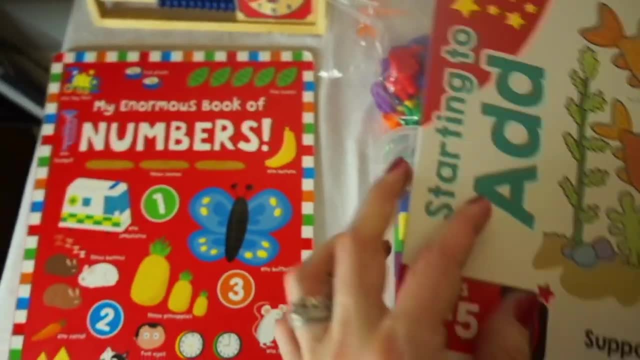 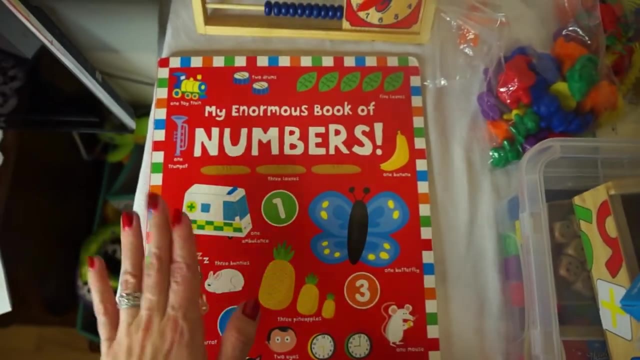 I've also got the starting to add one, which is actually quite simple, and then it goes on. it progressively gets a little bit more difficult towards the end. now, if you're just introducing numbers to your children. I've had this book for a long time. this is my enormous book of numbers. I've 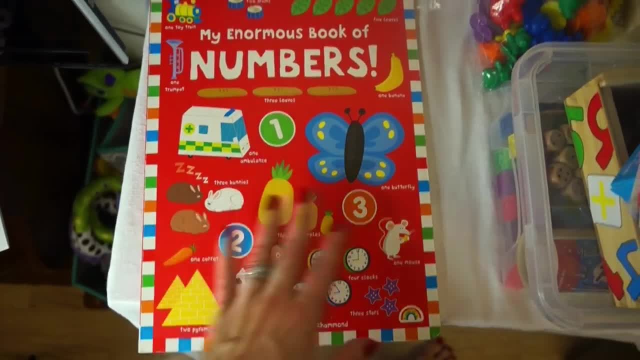 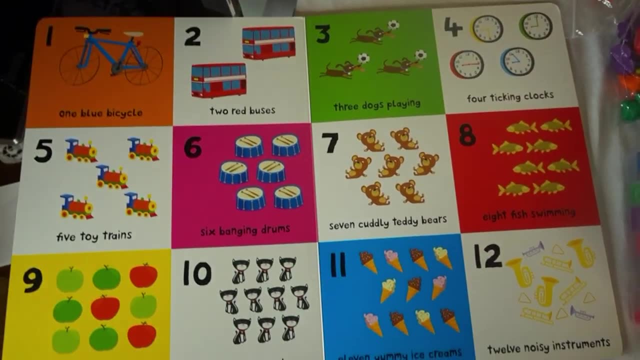 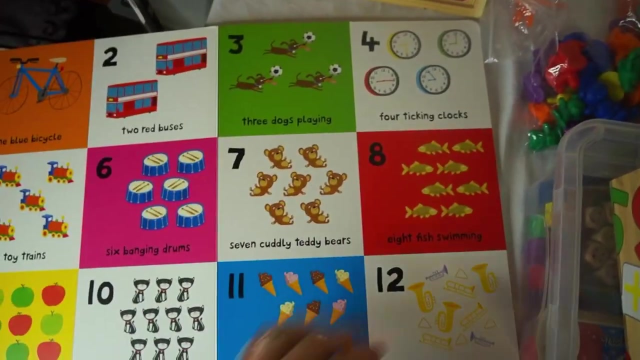 also got the my enormous book of colors and I think this is fantastic. it's really beautifully illustrated and we read this quite a lot actually, as, like our nighttime story, the children like saying: was one bike, how many bears? can they find the fish? and this is like a really nice introductory. 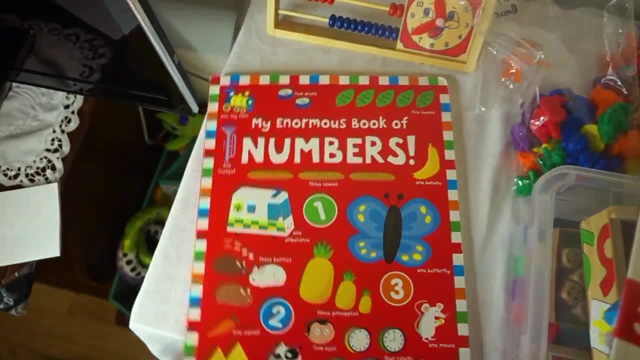 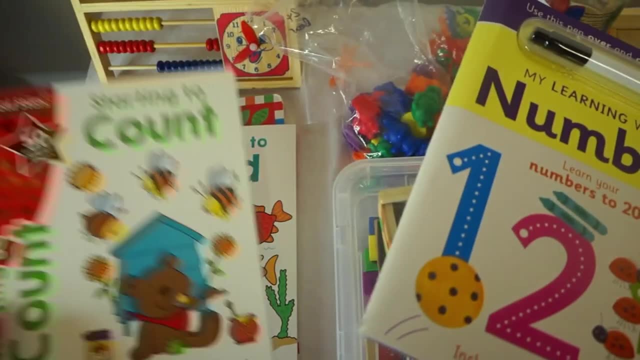 board book again, there are lots of board books out there with numbers. we've got lots of other books that have got numbers 1 to 20 in, or can you find the number and all that you'll find loads out there. it just depends on really what you want. 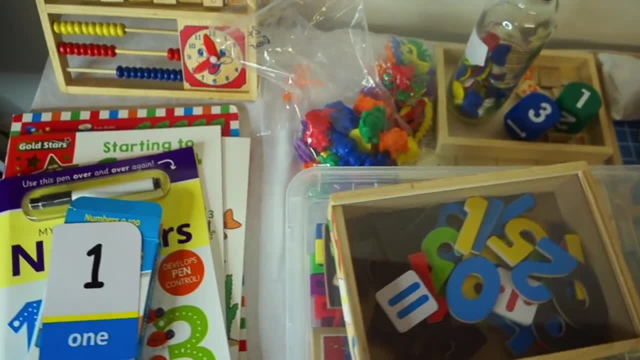 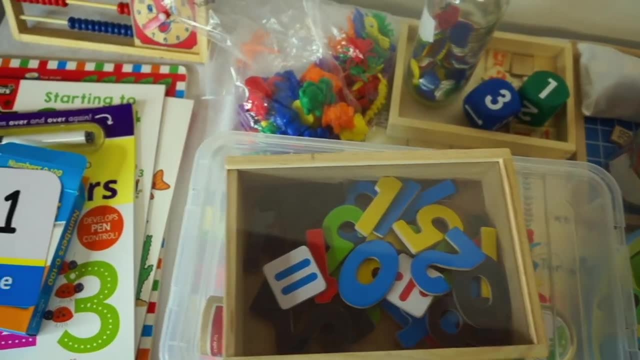 so there you go, guys. that was most of my mathematical and counting tools and materials. I've got my learning folders. I've got lots of educational games as well, but these were the basics, so I'll leave all the links down below. really hope you enjoy the video and look out. 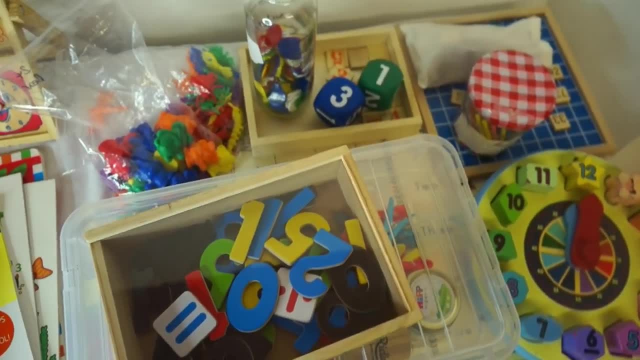 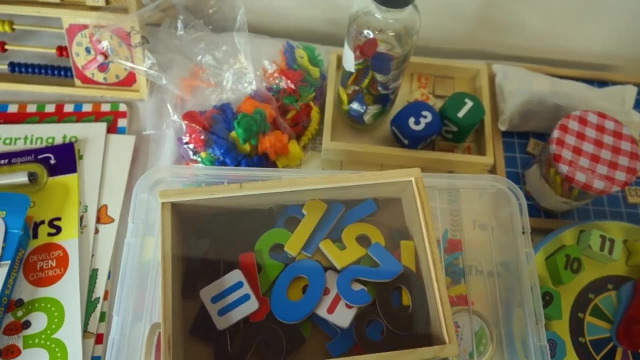 for my literacy learning materials and tools and things that I use for learning the alphabet and so on. that's coming very soon, so don't forget to subscribe if you like my content and hit that like button, and I shall see you next time. bye-bye.